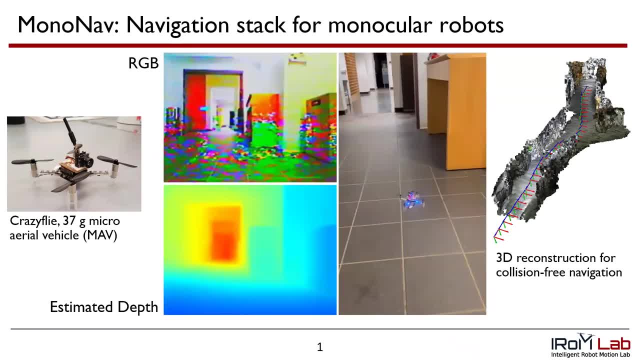 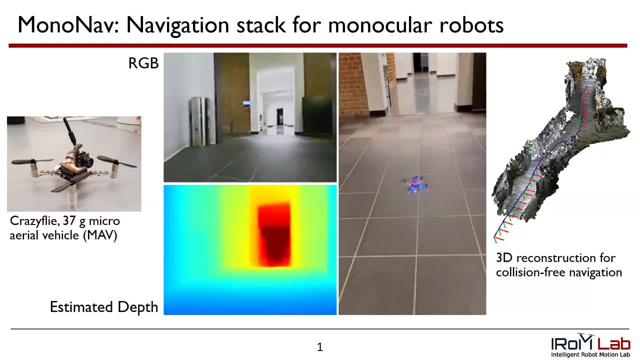 at 0.5 meters per second in a hallway environment. All the videos of MonoNav are shown in real-time. nothing is sped up. The per-frame metric depth estimation enables online 3D reconstruction, giving the MAV a map for online path planning. To our knowledge, MonoNav is the first monocular 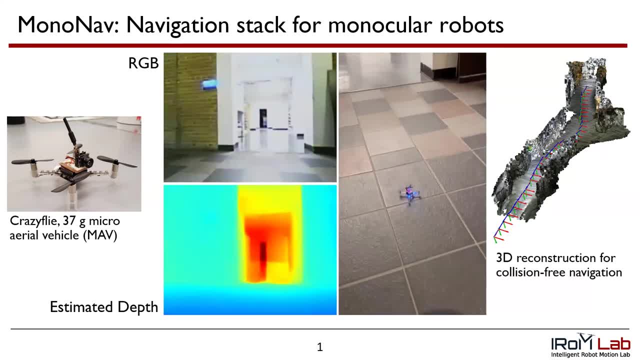 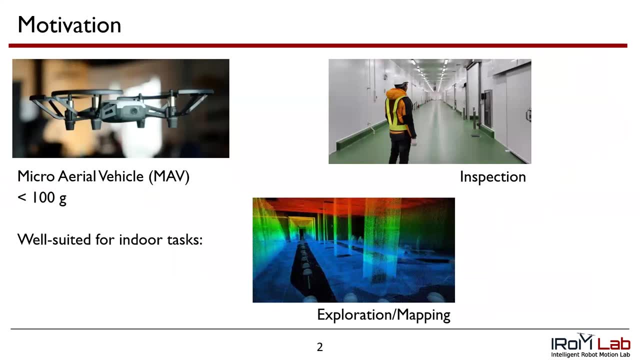 navigation stack implementation with distinct mapping and planning stages, evaluated in hardware. We test MonoNav in 15 different hallway environments, demonstrating its effectiveness in navigation. The smallest class of unmanned aerial vehicles, micro-aerial vehicles or MAVs, are well-suited for tasks such as inspection, exploration. 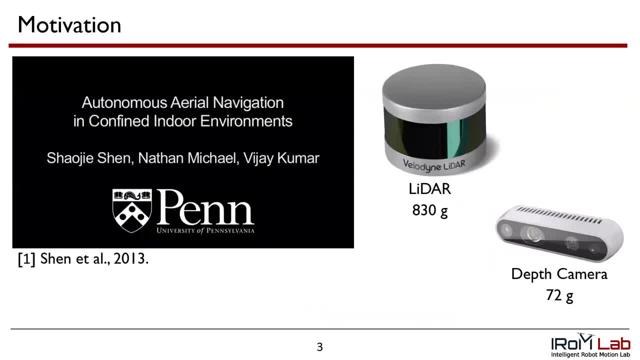 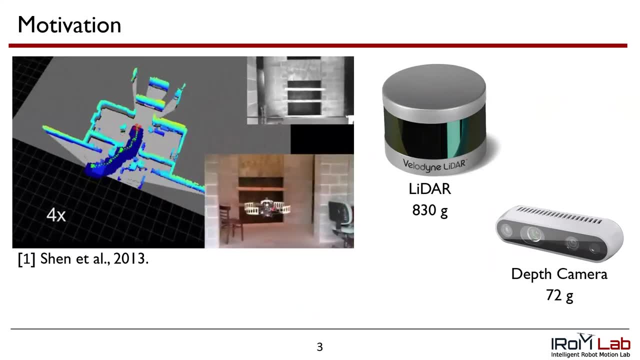 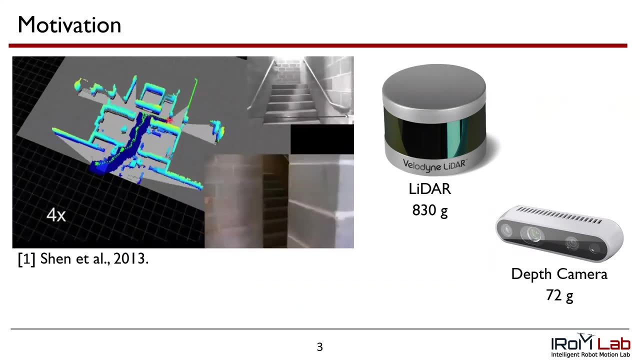 and mapping in constrained indoor environments due to their small size. When a robot has access to a local map, conventional path planning and trajectory optimization approaches can be used for collision-free navigation towards a goal. To generate such a map, online robots typically use depth sensors such as laser range scanners, LiDAR sensors or stereo. 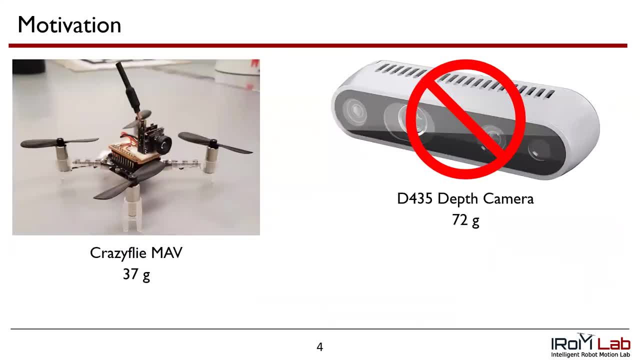 depth cameras to sense the local positions of obstacles. These depth sensors are far too large to be integrated onto a MAV, which typically only has access to its pose and a front-facing RGB camera For this problem. while all sensing is on board, we assume that the MAV 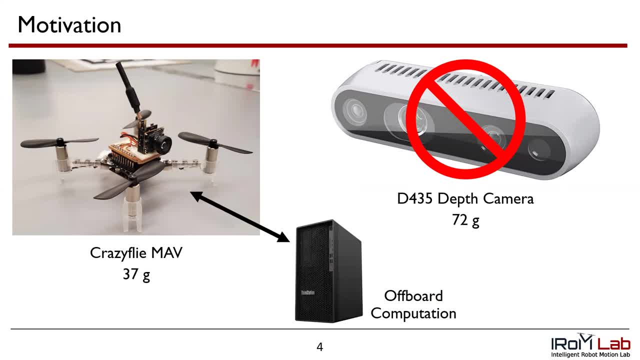 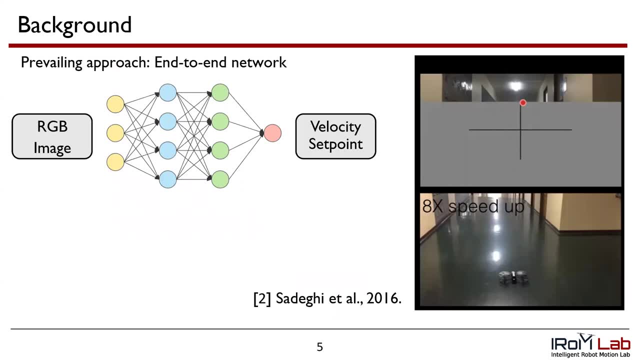 has access to an off-board computer, for example a desktop. The prevailing approach for MAV navigation without depth sensors is to use a learned end-to-end model which maps an input image to a velocity command. In this video, a model trained entirely in simulation can 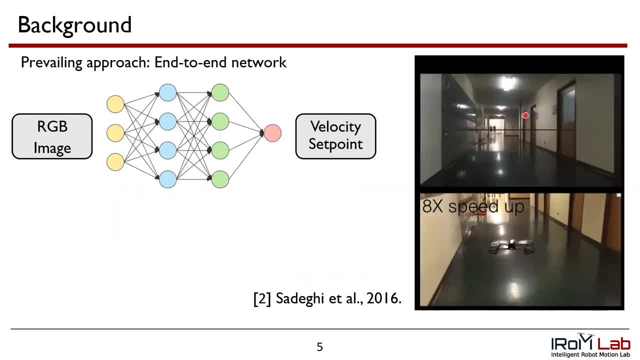 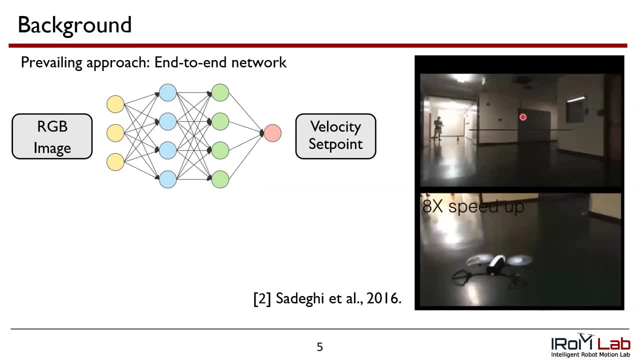 successfully navigate indoor environments. The downside to these approaches is that the MAVs are not designed to be used as a model. A specific model may not generalize broadly to unseen environments or conditions. In addition, tweaking the objective or desired behavior may require retraining the model entirely. If the MAV had access to a map instead, the user would have more. 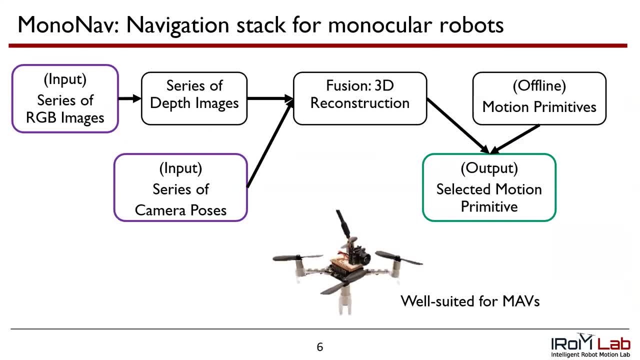 flexibility in planning and control. To that end, we present MonoNav, a navigation stack for monocular robots. We start by taking a series of RGB images and camera poses which are readily available from the MAV. We then convert the RGB images into metric depth estimates. We then fuse. 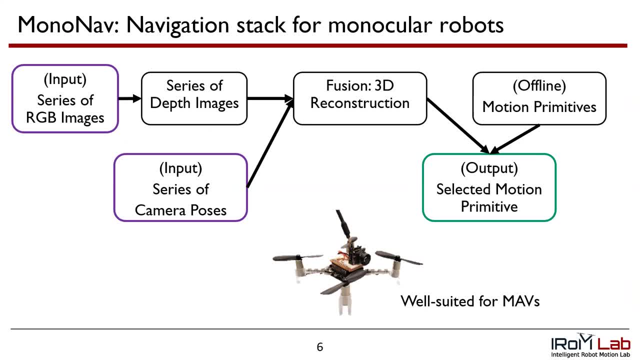 the poses and the depth of the model. We then convert the RGB images into metric depth estimates, into a 3D reconstruction that builds as the MAV moves through the scene. For planning we use motion primitives In principle, conventional path planning approaches such as RRT star or A star. 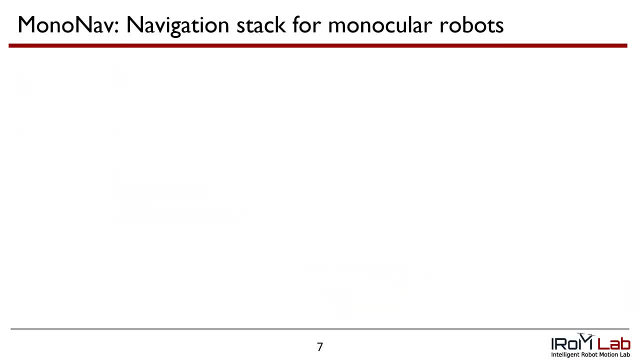 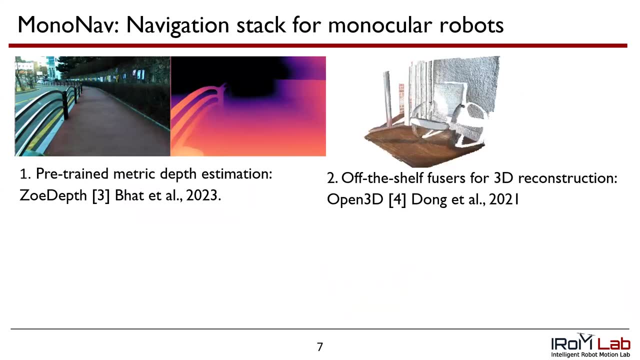 could be applied as well. We accomplish this by leveraging pre-trained transformer-based models for monocular depth estimation in combination with off-the-shelf and fusion and planning techniques. MonoNav uses ZOE depth for per-frame depth estimation and uses Open3D's tensor-based 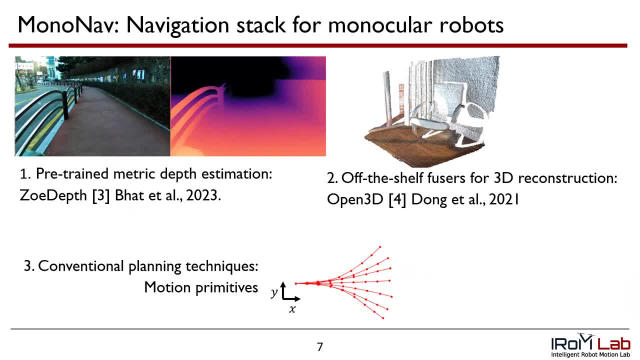 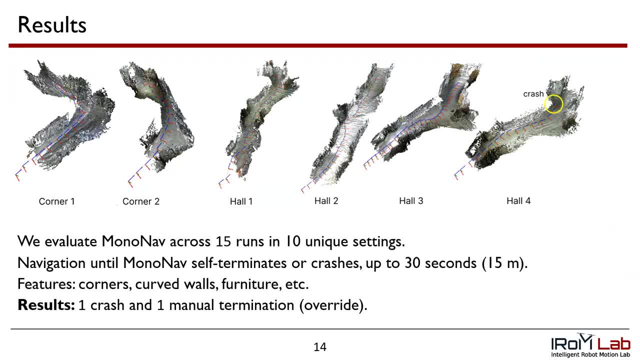 depth estimation. we use a pre-trained transformer-based model To determine the MAV's Navigation continues until MonoNav self-terminates or crashes up to 30 seconds or 15 meters. The hallway features are challenging, including corners, curved walls, columns and furniture. 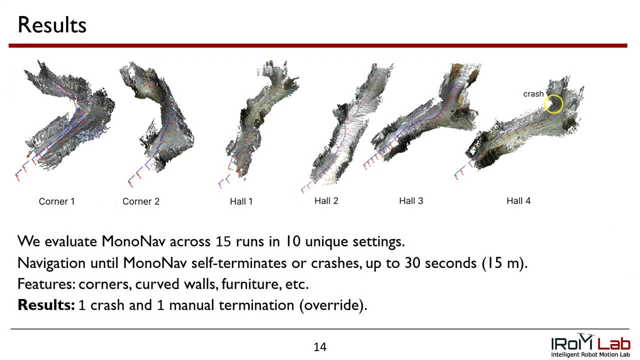 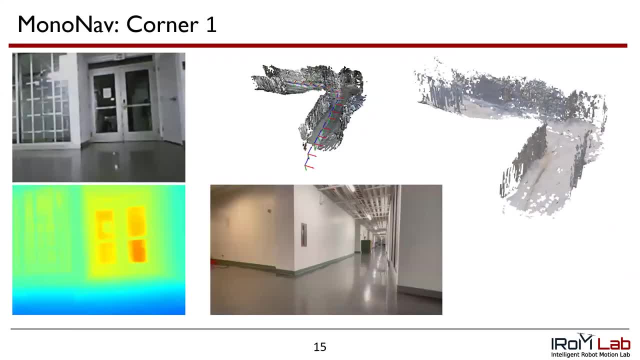 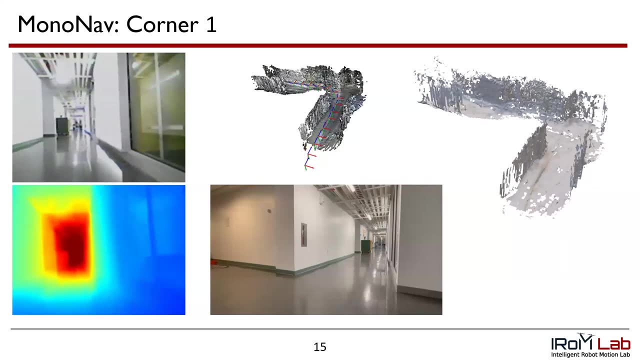 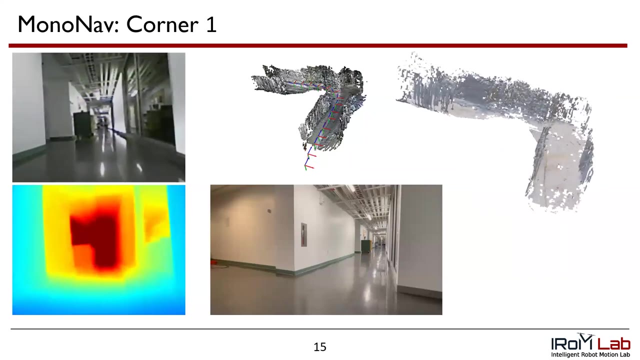 The results of MonoNav during the 15 runs are one crash and one manual termination. All others were self-terminations. Here is a corner example where MonoNav successfully navigates the corner. In another example, MonoNav navigates a long hallway straight. 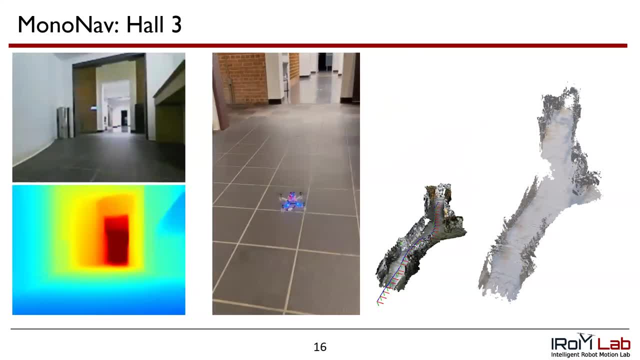 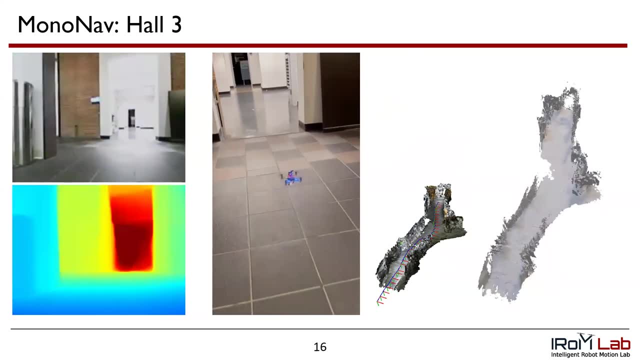 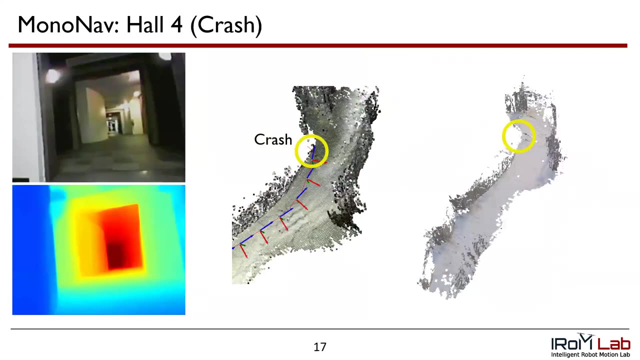 Here is a corner example where MonoNav successfully navigates the corner. Now we analyze the case where MonoNav crashed As the drone passes the curved wall on the left hand side, the same environment as in the previous reconstruction example. the wall occludes what lies beyond. 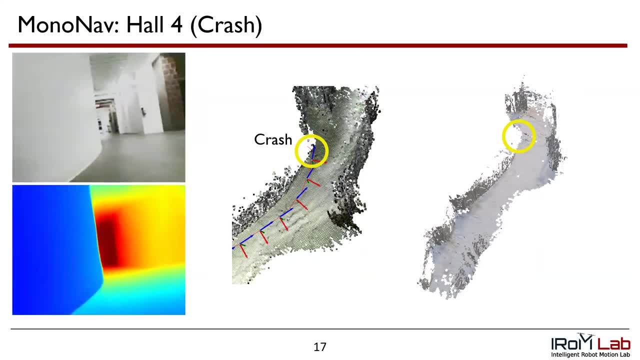 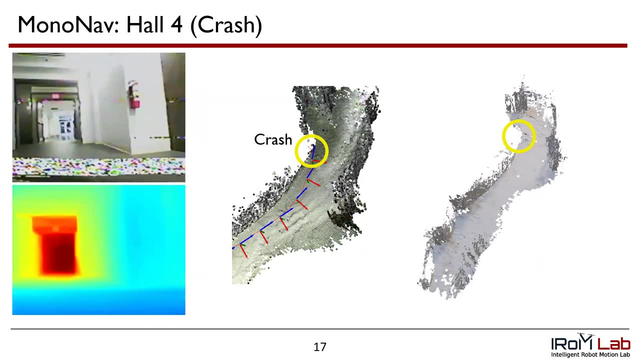 In addition, the smooth white curved wall surface is really difficult for ZoeDepth to analyze. As the drone passes the curved wall on the left hand side- the same environment as in the previous reconstruction example- the wall occludes what lies beyond a result the drone turns into what it thinks is empty space. This is a fundamental challenge. 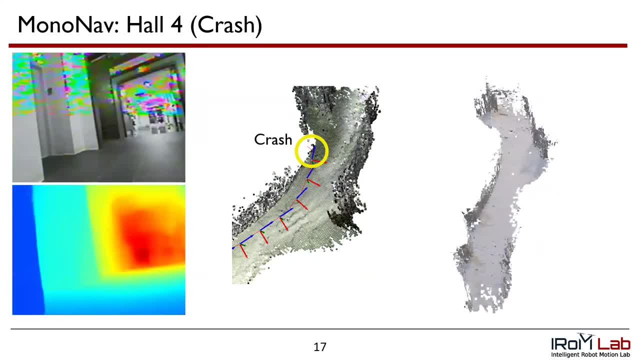 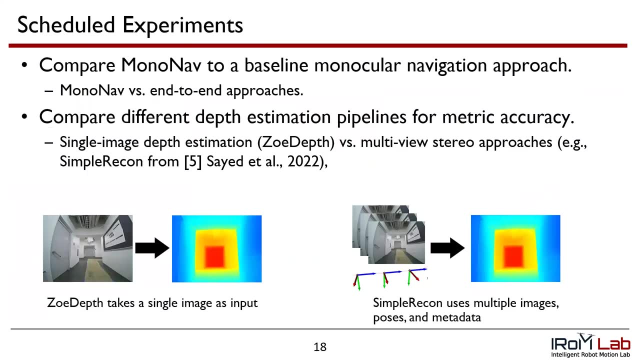 in monocular depth estimation, which could possibly be addressed by more cautious or slower primitives. We demonstrate MonoNav's performance in challenging indoor environments. However, we propose the following experiments to further evaluate MonoNav One: compare MonoNav against a baseline monocular navigation approach, such as state-of-the-art end-to-end navigation. 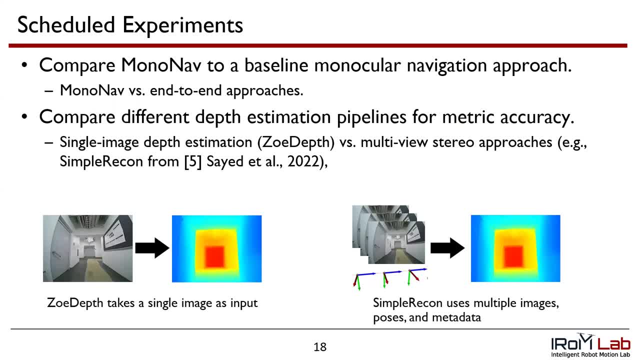 And two compare reconstruction quality against baseline depth estimation pipelines. MonoNav uses ZOE depth, which infers depth from a single image. Other methods, such as simple recon, use a series of frames, poses and metadata to infer depth. Such multi-view stereo approaches.